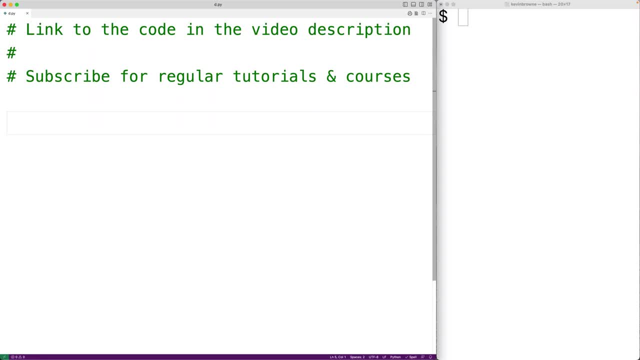 In this video we're going to learn how to find the smallest number in a file using Python. So if we have a file like this with one number per line of the file, what we want to do is find the smallest number in that file. The first thing we'll do is prompt the user to enter. 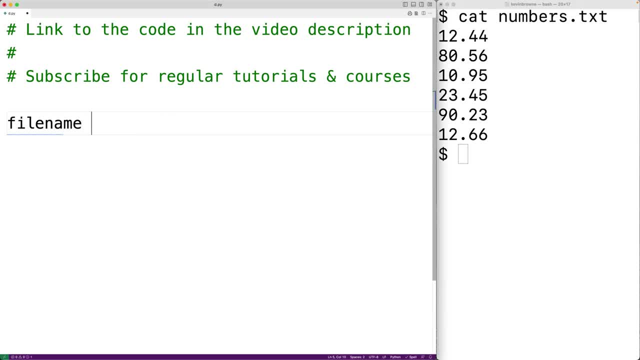 the file name. So we'll have here file name is equal to, and we'll call the input function and we'll pass it the string file name colon. This will prompt the user with that text. When the user enters the file name and hits enter, that string is going to be stored into file name. 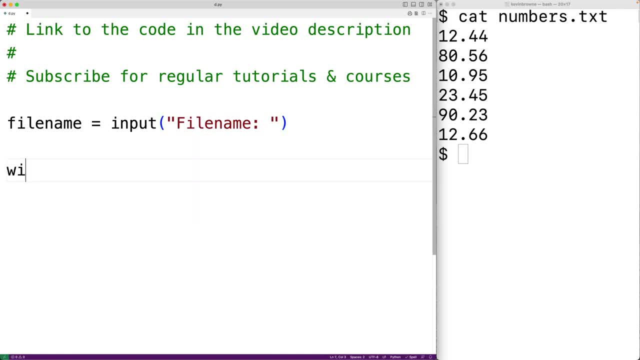 We can then open the file with that file name We'll have here with open file name as file. This is going to open the file with that file name, and file is going to be a file object which will allow us to read the file. 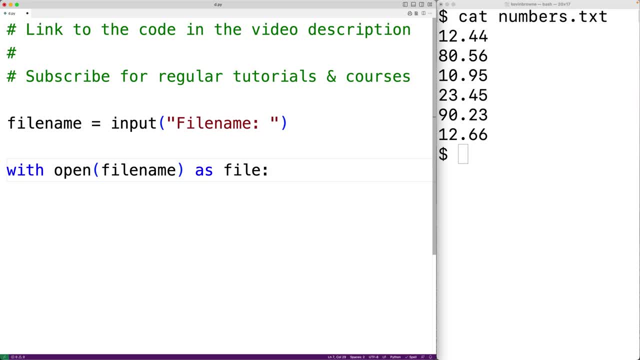 We can then use the read lines method of the file object to read the file contents. So here we'll have lines. list is equal to and we'll have file dot read lines. So read lines is going to return each line of the file stored as a string in a list. 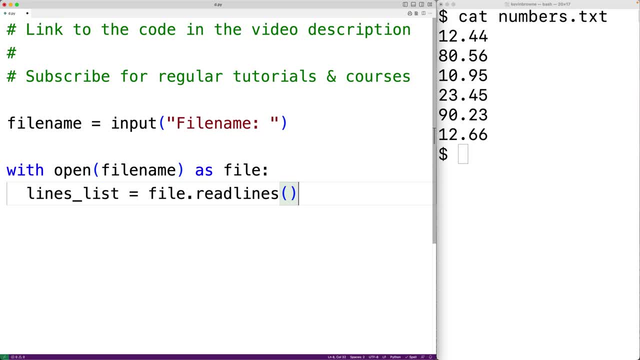 So lines list is going to be a list containing each line of the file as a string. We could actually output that list. We'll have here print and then lines list. We'll save our program and we'll run it and we'll enter in the file name. 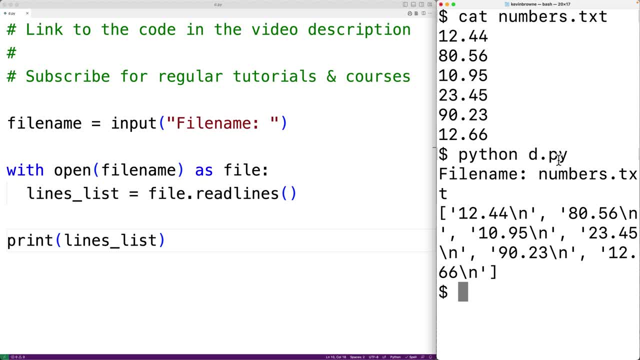 numberstxt and we can see. we get a list with each number in the file stored as a string. What we want to do is find the smallest number in the file. We'll need to convert these strings to float values. We'll do this using a list comprehension. We'll have here float underscore list. 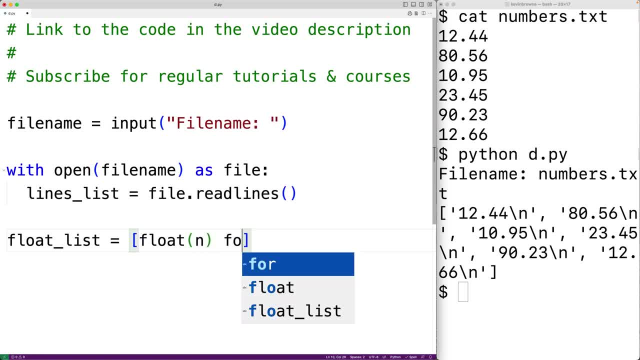 is equal to and we'll have float n for n in lines list. So this is a list comprehension. We're going to use lines list to make a new list. So for each string element n in lines list, float is going to be applied to the element. Float is going to return the floating point number.